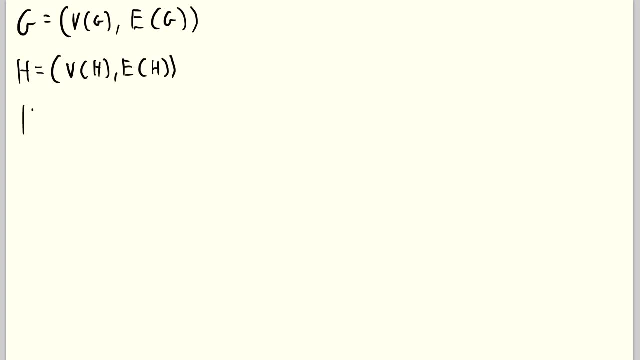 and edge set E of H, Then H is a subgraph of G written like this, using the same notation as we use for subsets: H is a subgraph of G if and only if, which I'll abbreviate with the if with two Fs. So H is a. 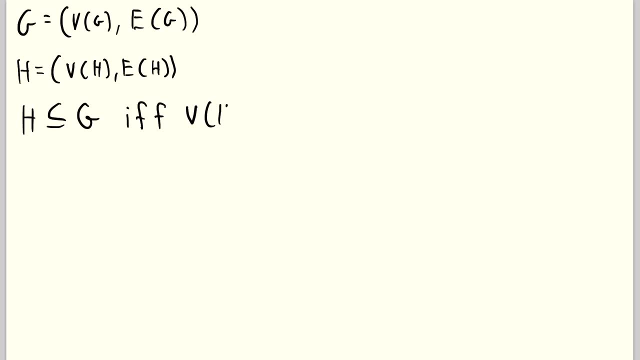 subgraph of G if, and only if, the vertex set of H is a subset of the vertex set of G and the edge set of H is a subset of the edge set of G. And rather than using the comma there, I'll use the. 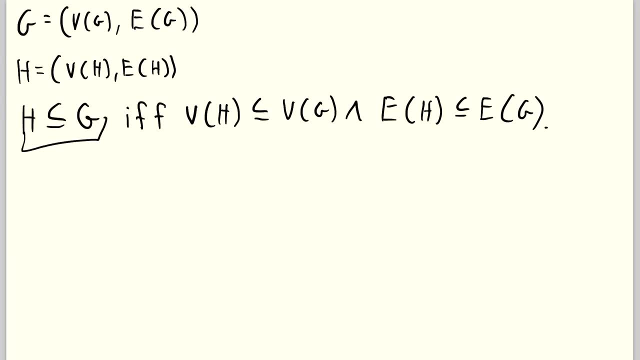 symbol. that means: and So H is a subgraph of G if, and only if, the vertex set of H is a subset of the vertex set of G and the edge set of H is a subset of the edge set of G. So all of that just means that H is a subgraph of G. 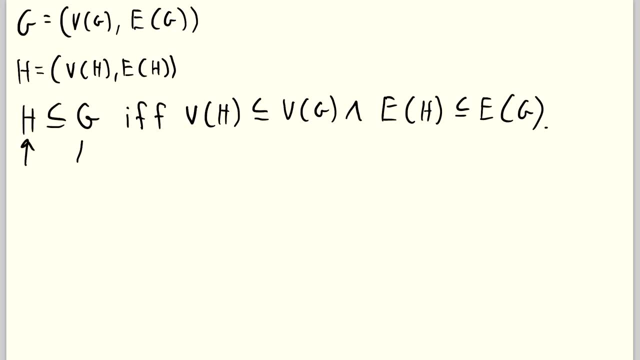 if, and only if, everything in H is also in G. So if H has something in it that G doesn't, then H is not a subgraph of G, but if G has in it everything that is in it, then H is a subgraph of G. 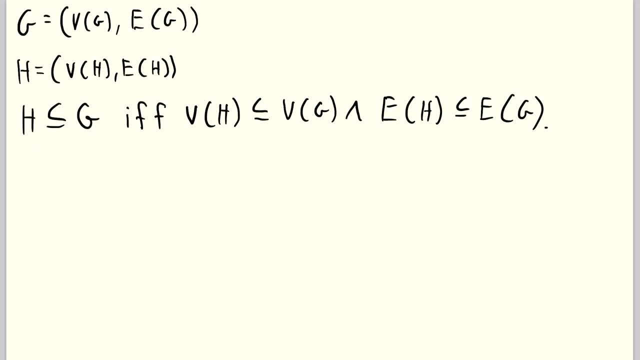 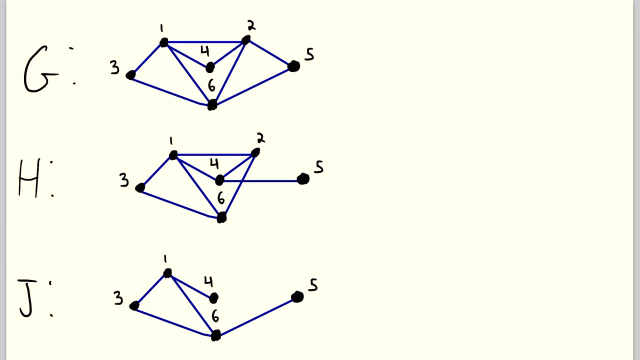 So now let's look at some graph diagrams. So here we've got three graphs- G, H and J, And the question I'll present to you is which one of these two graphs, H or J, is a subgraph of the graph G? 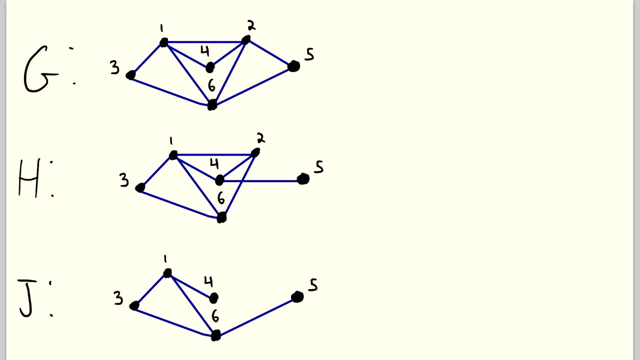 So all we have to do is look at the two graphs, H and J, and see which one has vertices and edges which are all in G, and which one has a vertex or an edge that isn't in G. Let's start off with H. So if we look at H, let's look at its vertex set first. In its vertex set it has: 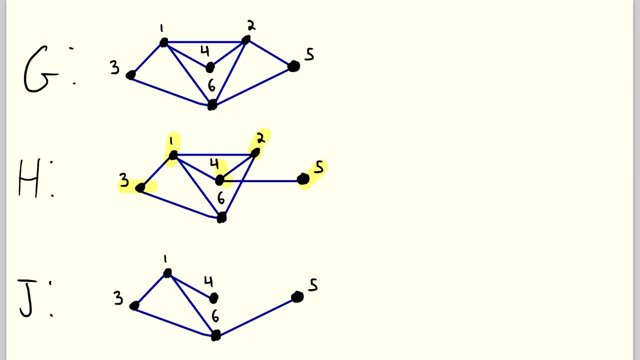 1,, 2,, 3,, 4,, 5, and 6.. And that is the same vertex set as G. G also has the vertices 1,, 2,, 3,, 4,, 5, and 6.. 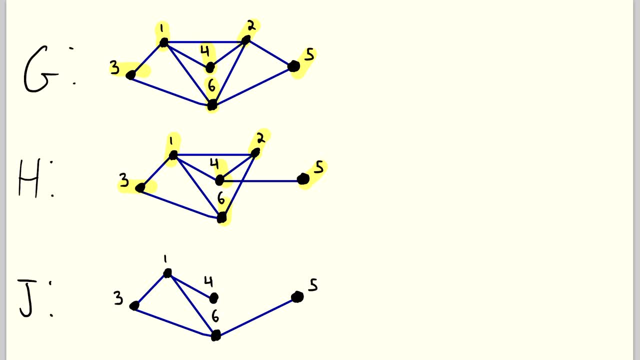 So the vertex set of H is a subset of the vertex set of G. It happens to be equal to the vertex set of G, but that is still a subset by definition. So then we'll move on to the edges, and I'll highlight the edges. 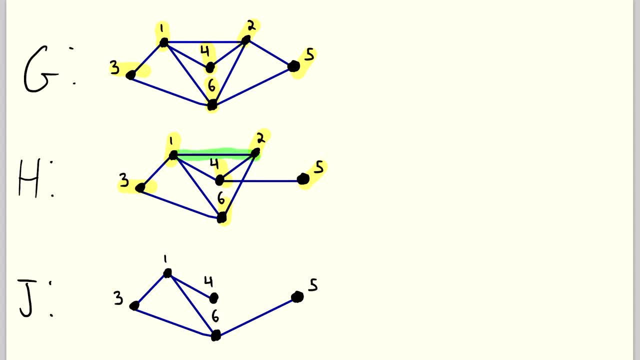 in green. So we see that 1 and 2 are joined in H. They're also joined in G. 1 and 4 are joined in H. They're also joined in G. 2 and 4 are joined in H. They're also joined in G. 4 and 5 are joined in H. 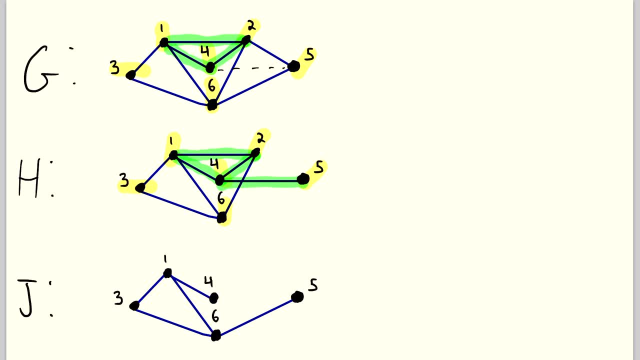 And we see that 4 and 5 are not joined in G. Thus we can conclude that H is not a subgraph of G because H contains an edge, the edge that joins 4 and 5.. That is not in G And that's all we need is one thing in H that isn't in G, to say that H is not a subgraph of G. 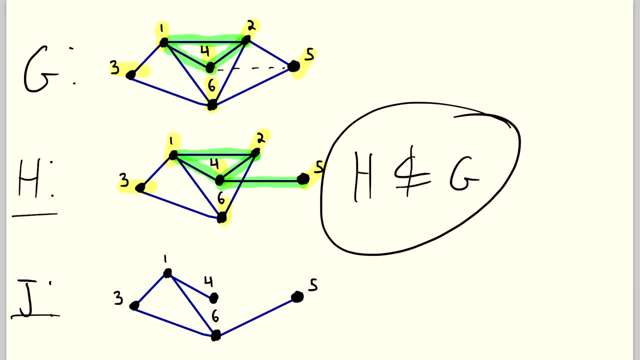 So then, because one of these two graphs is a subgraph and one isn't, that leads us to conclude that J is a subgraph, but let's take a closer look at it to find out why. So again, we'll look at the vertex set. 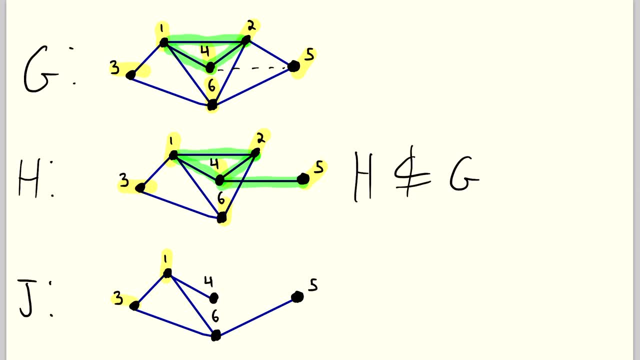 And J has vertices 1,, 3,, 4,, 5, and 6.. And we already know that all of those vertices are also in G. So so far, so good. And then again I'll highlight in green, We'll look at the edges. 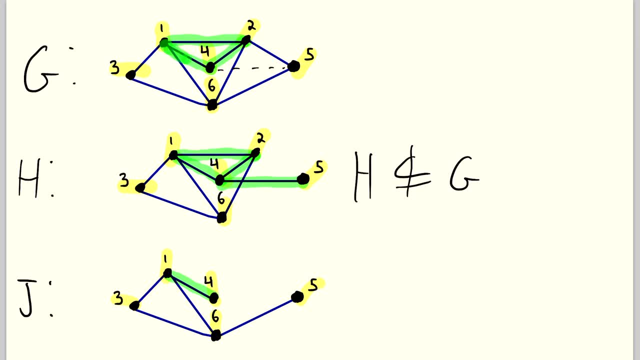 1 and 4 are joined in J. We see that those are also joined in G. 1 and 6 are joined in J, as they are also in G. 1 and 3 are joined in J. They're joined in G. 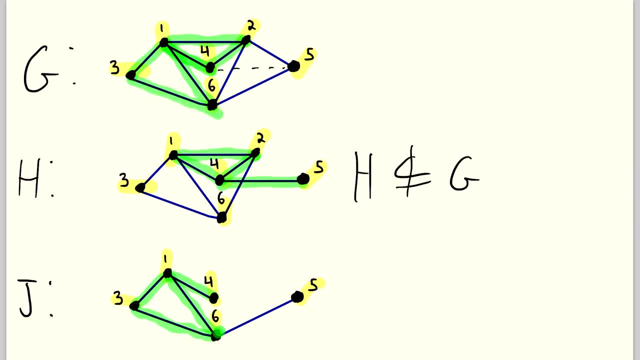 3 and 6 are joined in J. They're also joined in G. 6 and 5 are joined in J. They're also joined in G. And right, there is enough now to conclude that H is a subgraph of G, because every vertex in J that we looked at was in G. 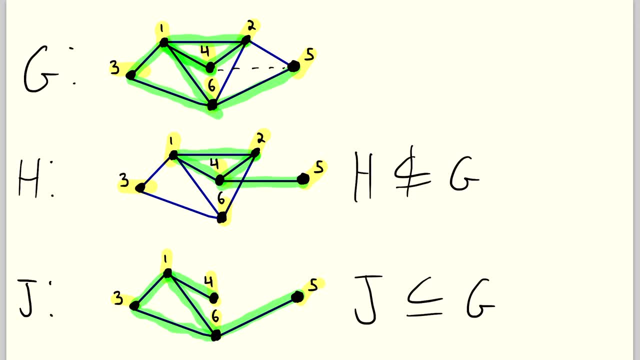 and we saw that every edge in J is in G. Thus J is a subgraph of G. Now if we were to add, let's say, an extra vertex to G, Let's say we add the vertex 7.. That doesn't change anything, right? 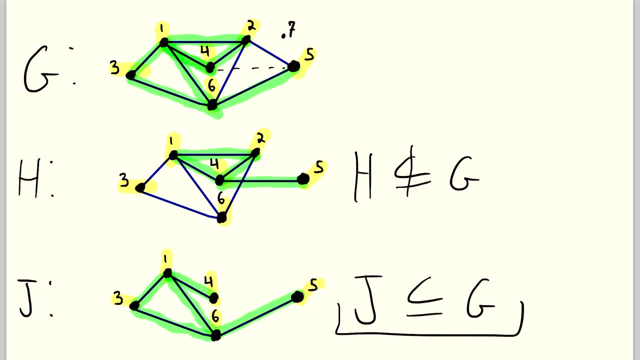 J is still a subgraph of G because everything in J is still in G. So we can add stuff to G and J will still be a subgraph of G. But if we were to take this vertex 7 and add it to J instead of G,